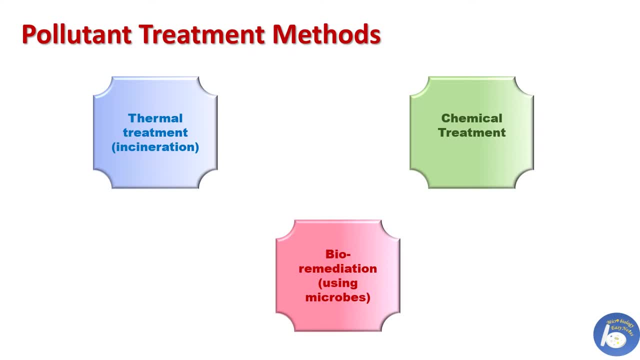 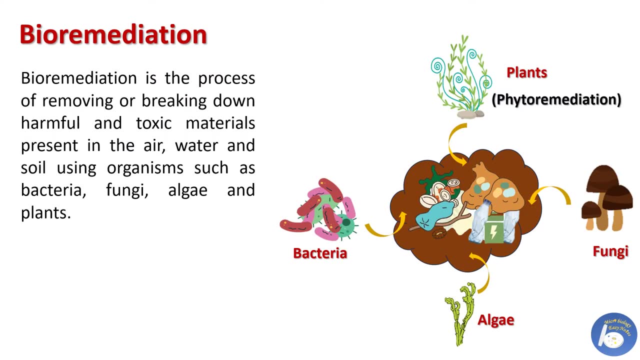 microbes are such methods. This video is about bioremediation, so we will focus on that. What is bioremediation? It is the process of removing or breaking down harmful and toxic materials present in the air, water and soil, using organisms such as bacteria, fungi and plants. 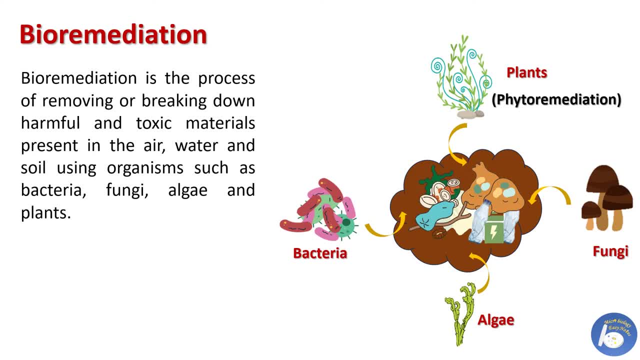 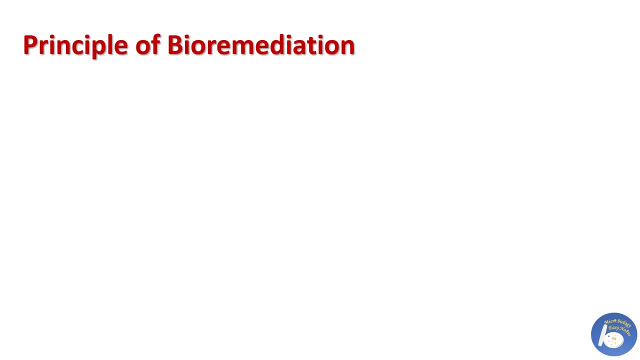 If the plants are involved, process is called phytoremediation. If bacteria, fungi, yeast, algae and actinomyces are involved, it is known as microbial remediation. Principles behind bioremediation: microbes exist which eat and digest toxic materials like xenobiotics, plastics. 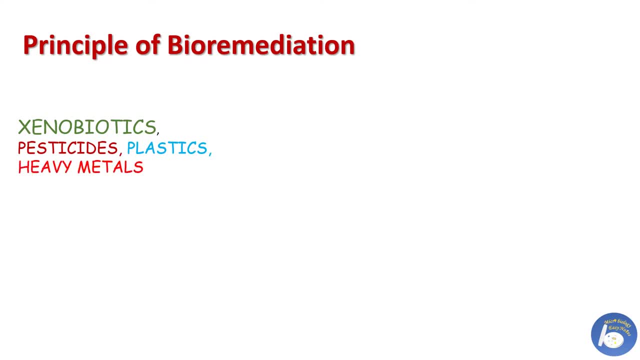 pesticides and heavy metals, etc. and convert them into less toxic or non toxic substances such as water and gases like carbon dioxide and ethane. these microbes have genetic machinery and certain enzymes that they can easily degrade harmful compounds. watch my video on xenobiotics: link in the comment. 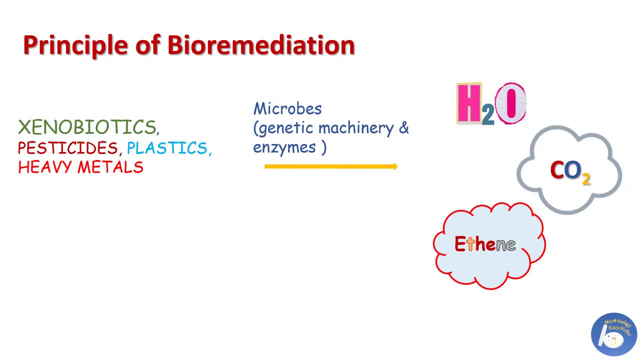 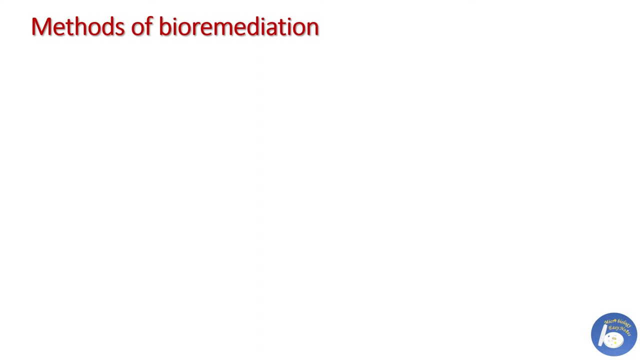 section. moreover, microbes have capability to adjust themselves as per surroundings. therefore they can work on extreme sites also, and these qualities are helpful for pollutant degradation. methods of bioremediation: there are many bioremedial techniques available, but basic methods can be one of them. behind those techniques, first is natural. 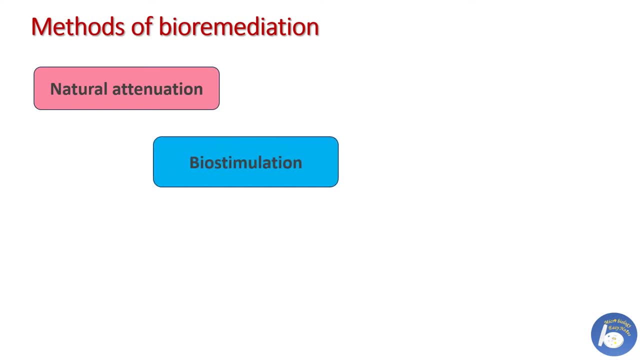 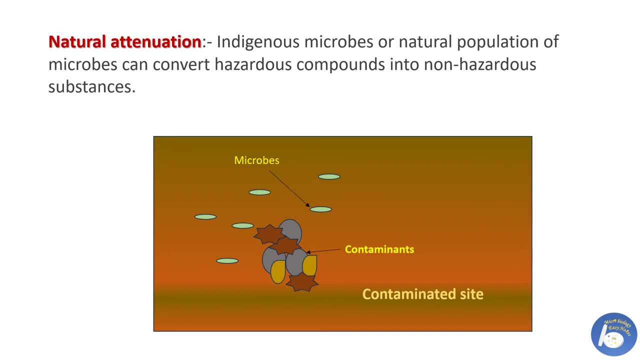 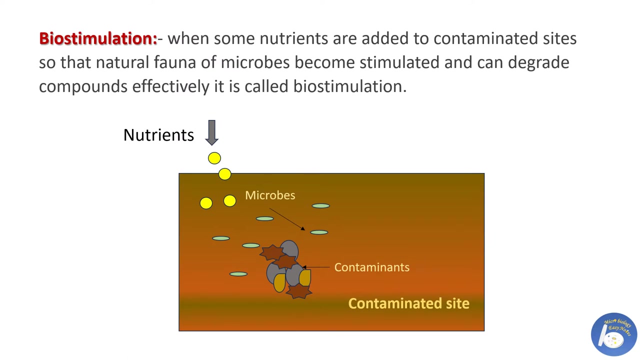 attenuation, second is biostimulation and third is Bioaugmentation. Natural attenuation: Indigeneous microbes or natural population of microbes are able to convert hazardous compounds into non-hazardous substances. then process is called natural attenuation. Biostimulation: Some nutrients are added to contaminated site so that natural mona of microbes become stimulated and degrade compounds effectively. It is called biostimulation. 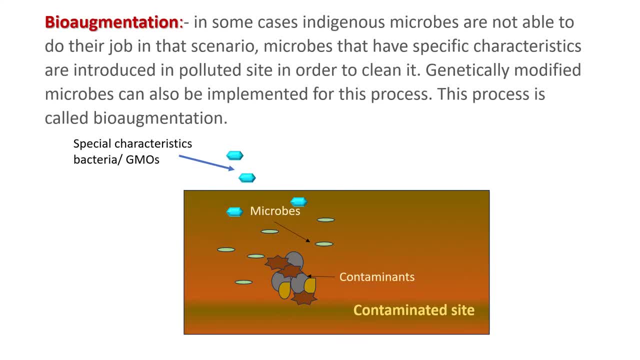 Bioaugmentation. In some cases, indigeneous microbes are not able to do their job. In that scenario, microbes that have specific characteristics are introduced in polluted site in order to clean it. Genetically modified microbes can also be implemented. Then the process is called bioaugmentation. 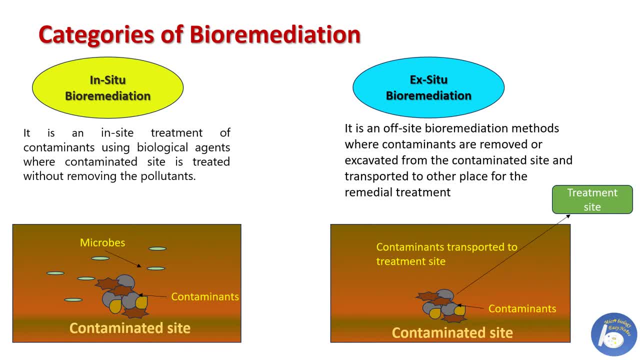 Categories of bioremediation. Majorly, there are two types of categories. First is in-situ bioremediation. In-situ means in the system. In-situ bioremediation is an in-site treatment of contaminants using biological agents where contaminated site is treated without removing the pollutants. 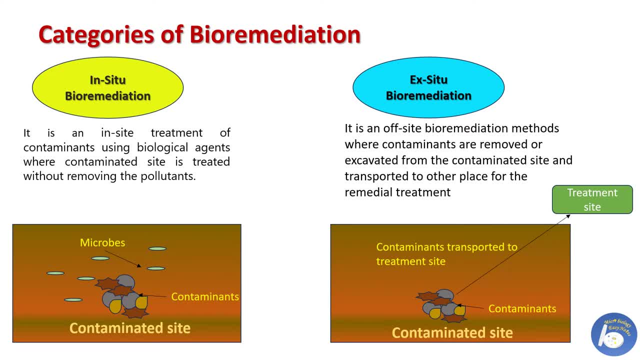 It is clean up. It is a clean up approach between microbes and the contaminants directly at the site, Ex-situ bioremediation. Ex-situ means outside the system. It is an off-site bioremediation method where contaminants are removed or excavated from the contaminated site and transported to other place for the remedial treatment. 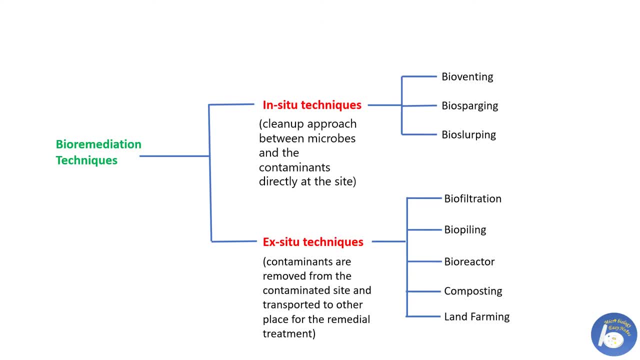 And now, what are the techniques involved in in-situ bioremediation and ex-situ bioremediation? In in-situ bioremediation, the techniques are bioventing, biosparging and bioslurping. In ex-situ, there are biofiltration, biopiling, bioreactor, composting and land farming. 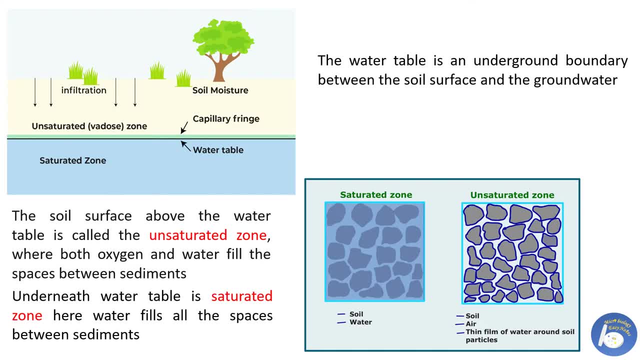 Before going into details of in-situ techniques and ex-situ techniques, we should know what is water table, unsaturated zone and saturated zone. The water table is an underground boundary between the soil surface and the ground water. Water pressure and atmospheric pressure are equal at this boundary. 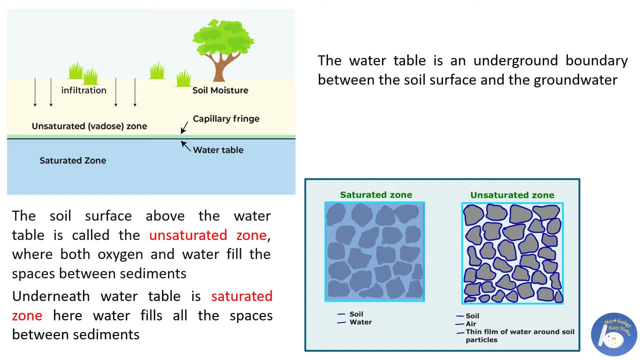 The soil surface above the water table is called the unsaturated zone, where both oxygen and water fill the spaces between sediments. Water is present as the thin layer around soil particles. Underneath the water table is the saturated zone. where water is saturated, Water fills all spaces between sediments. 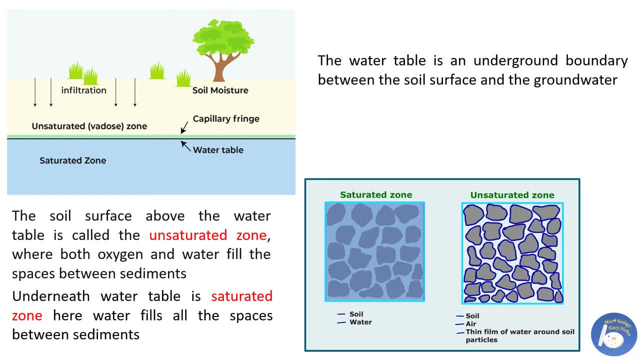 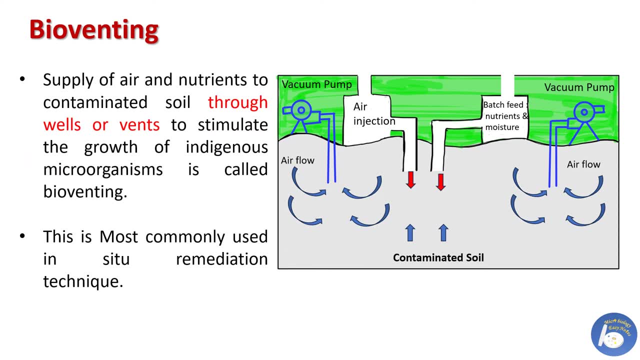 The saturated zone is bounded at the bottom by impenetrable rocks. And now we come to in-situ techniques. First technique is bioventing. Supply of air and nutrients to contaminated soil through wells or vents to stimulate the growth of indigenous microorganisms is called bioventing. 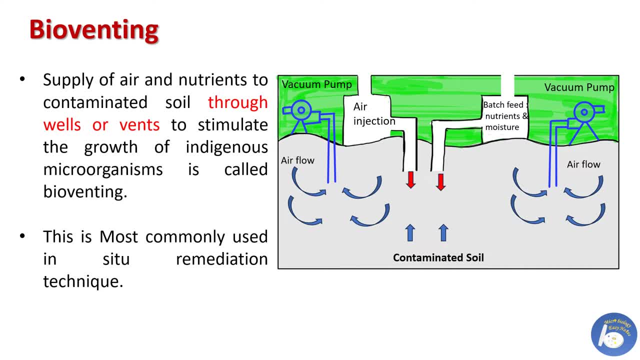 So what exactly happens in this process is, if enough nutrients and air are not present in contaminated site, we inject it via small opening which supports microbial degradation. This is the most commonly used in-situ remediation technique. This can be aerobic or anaerobic. 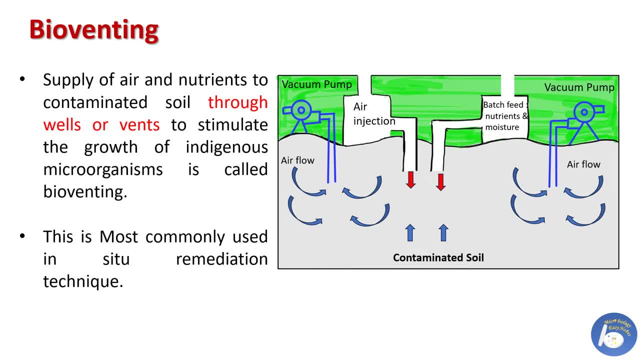 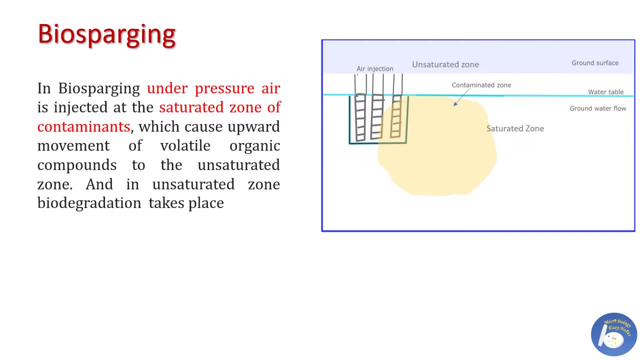 The process is employed to degrade simple petroleum hydrocarbons which are present far beneath the surface: Bio-sparging. In bio-sparging under pressure, air is injected at the saturated zone of contaminants, which cause upward movement of volatile organic compounds to the unsaturated zone. 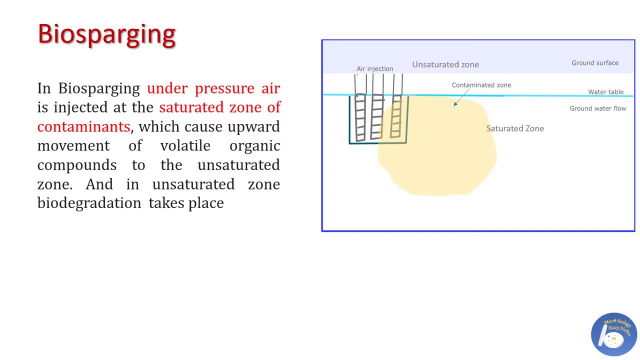 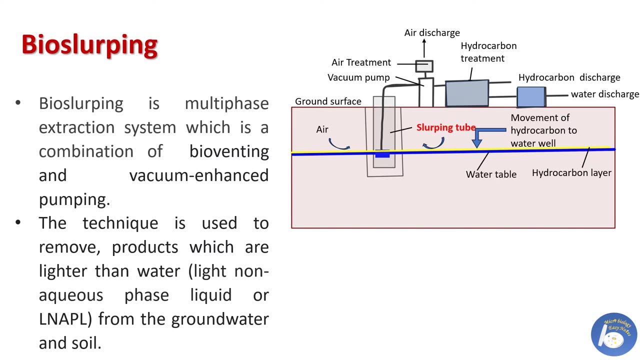 And in unsaturated zone, biodegradation takes place. This technique is used to reduce concentration of petroleum constituents that are dissolved in ground water. Bio-slurping- Bio-slurping is multiphase extraction system, which is a combination of bio-venting and vacuum-enhanced pumping. 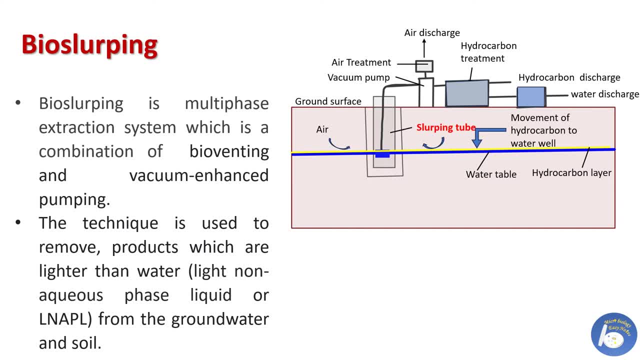 The technique is used to remove products which are lighter than water from the ground water and soil, These products also known as light non-aqueous phase liquid or LNAPL. The bio-slurper system uses a slurp tube that extends into the free product layer. 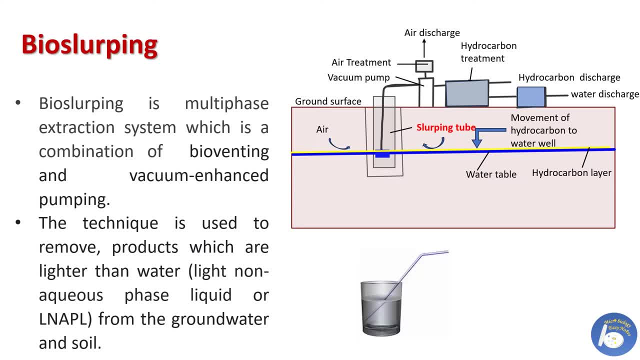 Much like a straw in a glass, draws liquid, the pump draws LNAPL. The LNAPL is brought to the surface where it is separated from water and air. Bio-slurping is limited to 25 feet below ground surface, as contaminants cannot be lifted more than 25 feet by this method. 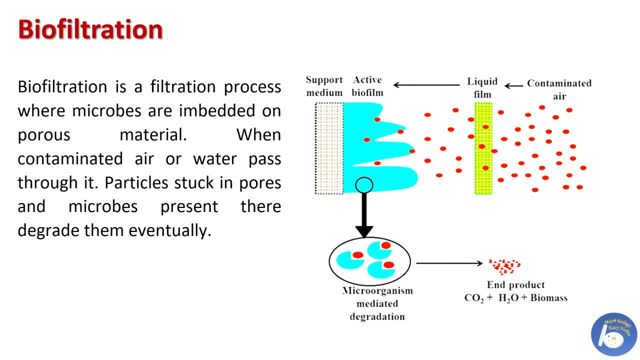 And now technologies involved in ex-situ bio-remediation. The first technique is bio-filtration. Bio-filtration is a filtration process where microbes are embedded on porous material. When contaminated air or water pass through it, particles stuck in pores and microbes present there degrade them eventually. 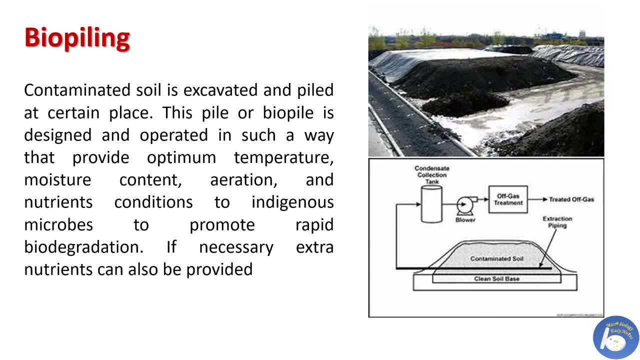 Bio-piling. In this process, contaminated soil is excavated and piled at certain place. This pile, or a bio-pile, is designed and operated in such a way that provide optimum temperature, moisture content, aeration and nutrient condition to indigenous plants. 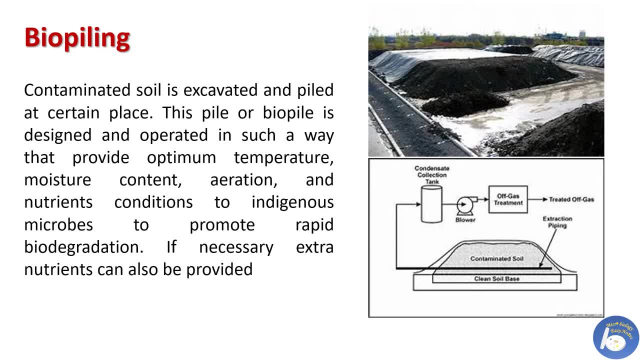 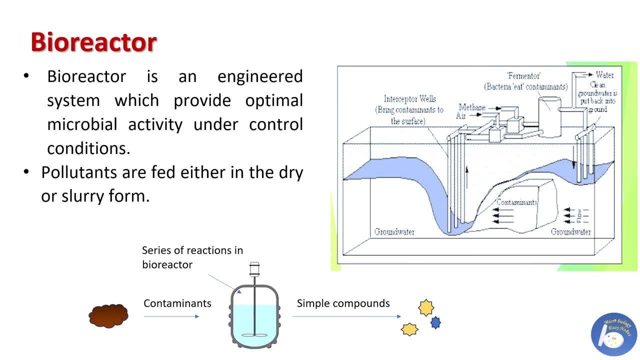 Bio-filtration is a process that allows microbes to promote rapid bio-degradation. If necessary, extra nutrients can also be provided. Bio-reactor- Bio-reactor is an engineered system which provide optimal microbial activity under controlled conditions. Pollutants are excavated from the site and fed into bio-reactor vessel. 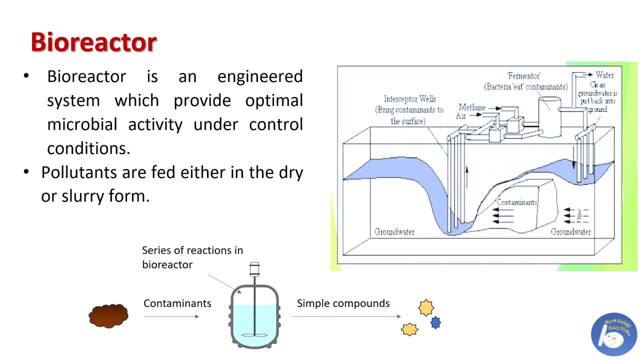 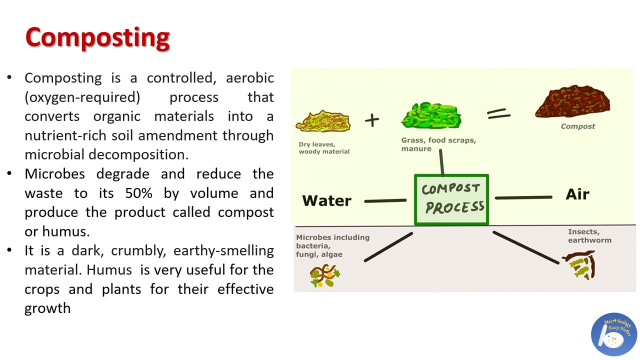 where series of biological reactions and microbial activities degrade these contaminants. Pollutants are fed either in the dry form or slurry form. Composting- Composting is a controlled aerobic process that converts organic materials into a nutrient-rich soil amendment through microbial decomposition. 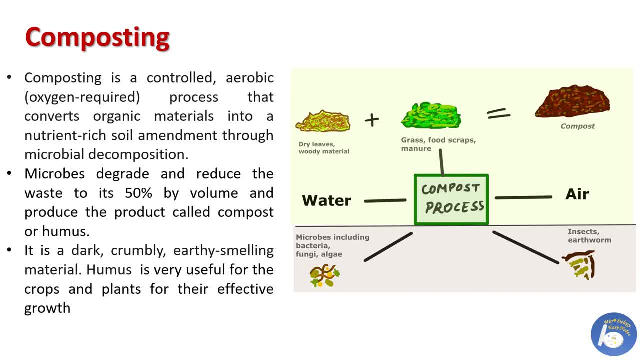 Microorganisms feed on the materials added to the compost pile during the composting process. They degrade and reduce the waste to its 50% by volume and produce the product called compost or humus. Humus is a dark, crumbly earthy smelling material. 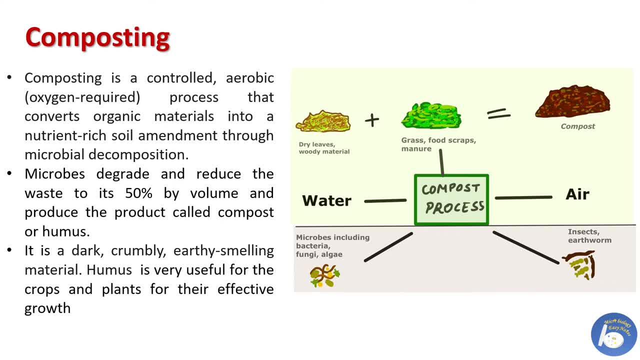 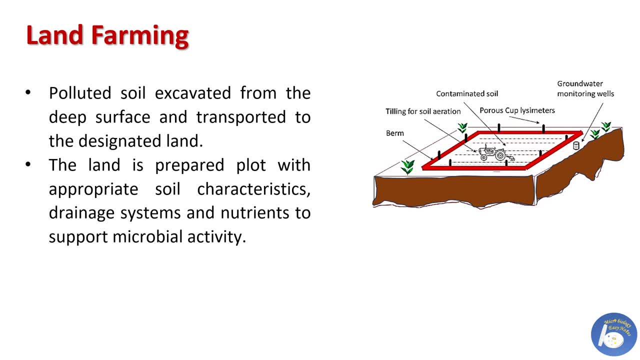 Humus is very useful for the crops and plants for their effective growth. Land farming: Land farming is solid-phase treatment process in which contaminated soil can be treated. Polluted soil excavated from deep surface and transported to the designated land. The land is prepared, plot with appropriate soil characteristics, drainage system and nutrients to support microbial activity. 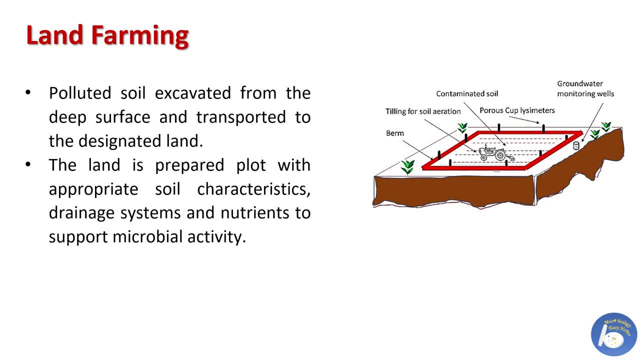 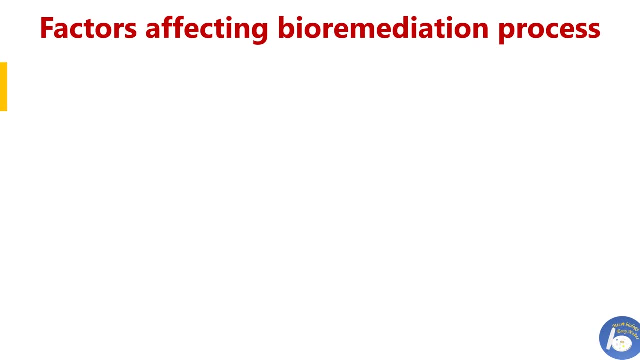 Land farming is a reliable process, but not suitable for highly volatile organic compounds and substances which are prone to bio-leaching. And now, what are the factors which can affect bio-domination process? First is concentration of contaminants. Higher concentration of contaminants takes longer time to degrade, while lower concentration of contaminants takes comparatively less time to degrade. 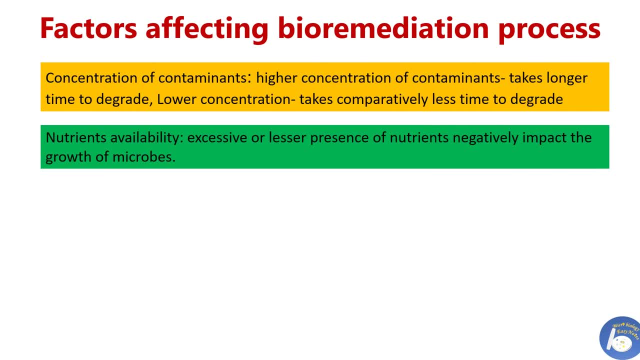 Second is nutrient availability. Second is nutrient availability. Concentration of nutrients directly affects the growth of microbes. Nutrients like carbon, nitrogen, phosphorus, potassium and calcium, etc. essential for the growth of microbes. Excessive or laser presence of these negatively impact the growth of microbes. 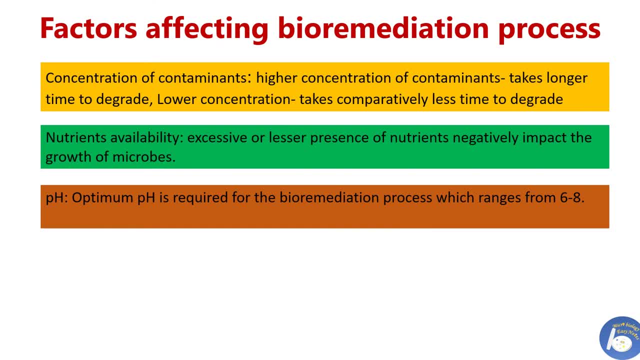 pH. Optimum pH is required for the bio-remediation process, which ranges from 6 to 8.. Neutral pH is suitable for the degradation of petroleum hydrocarbon, Whereas some fungi and acidophilic microbes degrade contaminants in an acidic environment. 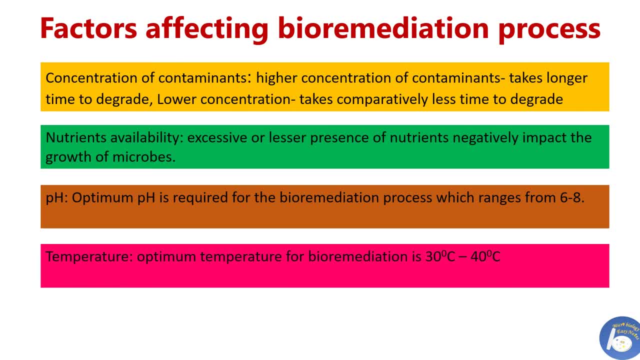 Temperature. Optimum temperature for bio-remediation is 30°C to 40°C. Next is oxygen. For aerobic bio-remediation, oxygen is required, while anaerobic bio-remediation process does not require oxygen. Aerobic degradation is much faster than anaerobic degradation. 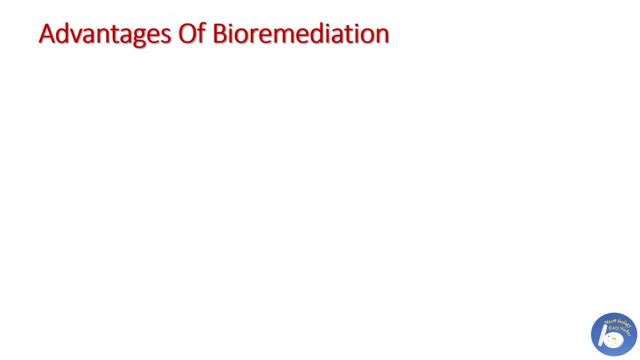 And also the process of bio-remediation is much more expensive than anaerobic process. Advantages of bio-remediation: First, it is cost-effective. Bio-remediation does not require expensive instruments, tools or equipment. 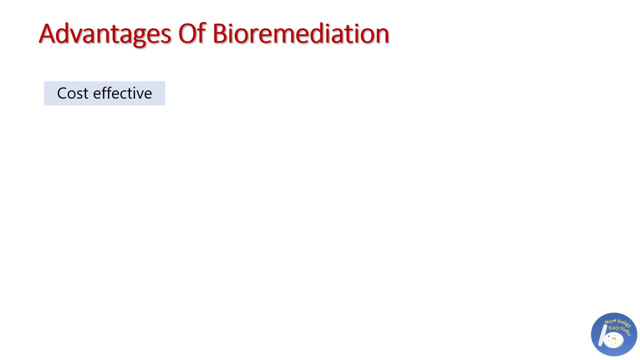 It can be performed inside as well, which reduce transportation cost. Energy consumption in this process is very low. Next is: this is environment friendly: This process is done by microbes that do not cause any harm of environment. Next is: this is environment friendly: This process is done by microbes that do not cause any harm of environment. 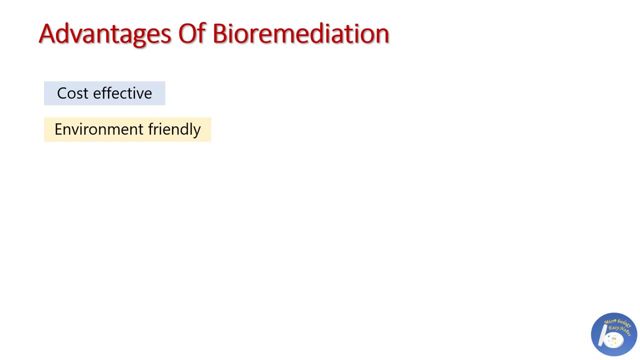 of environment: a light chemical method or use of incineration. next, it is versatile. bioremediation process can degrade wide variety of materials like pesticides, paints, petroleum, hydrocarbons, heavy metals and solvents, which can be applied on any environment like polluted air, soil or water. effectiveness: the effect of bioremediation lasts longer. it also reduces. 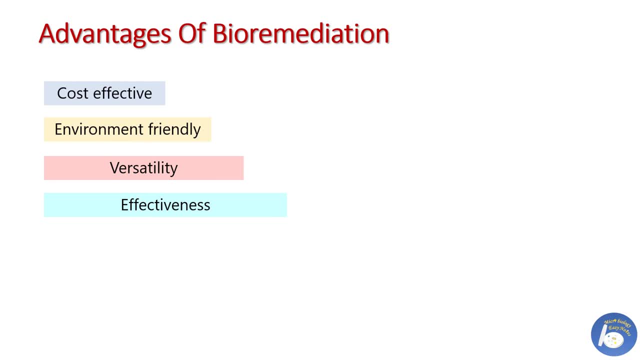 the future risk of recontamination. next, it is sustainable. it promotes the natural process of microbial degradation and plant assisted remediation, allowing ecosystem to recover and regenerate over time. minimum or no site destruction and disruption involved in this process. less human power is required. once the system is established, there is no need of 24 hours human workforce.